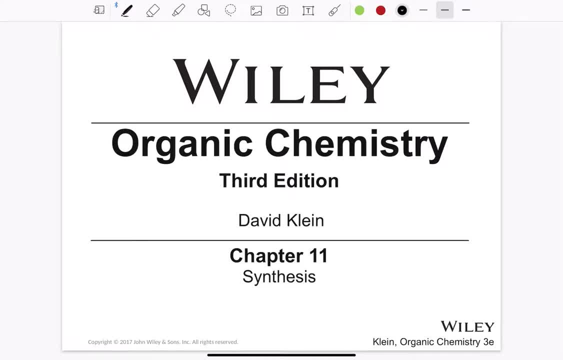 Hi guys, good day and hope you're well. So we discussed until now all the chapters that we discussed, all the lectures that we had. So we discussed different mechanisms and we also discussed different hydrocarbons. So in this chapter we'll try to coalesce everything and try. 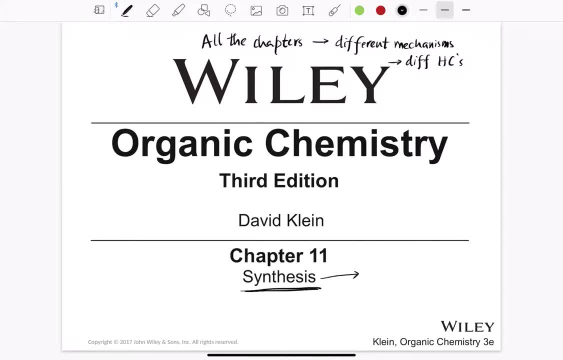 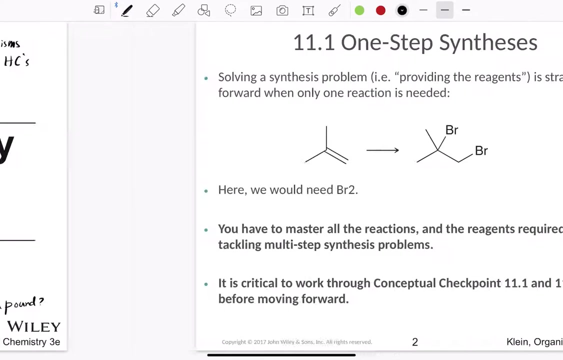 to come out as and talk about synthesis of compounds. So the chapter deals with. the main objective here is: how do you synthesize an organic compound? So this is the main question that we're going to answer in this chapter today. So if you look at a synthesis problem, the main question 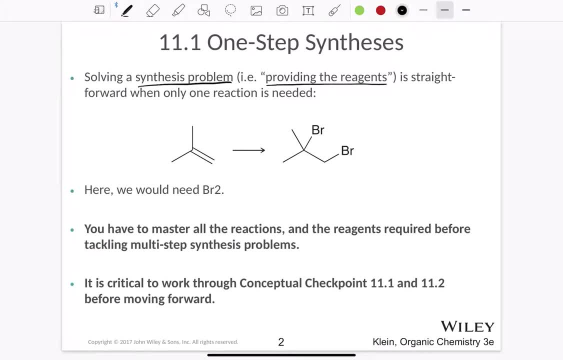 that we have is to understand what are the reagents that we need. If you have a single reaction, for example, let's say we have two propane and you want to produce 1,2-dibromopropane, So then we know that here we need. 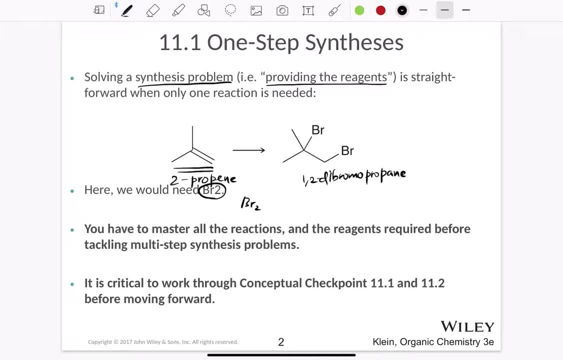 bromine, Br2.. So in this compound reduction here in the process that we are producing, we know that we need Br2.. The question comes back that how do you synthesize this compound? So to understand how to synthesize this, we must master all the reactions that are generally. 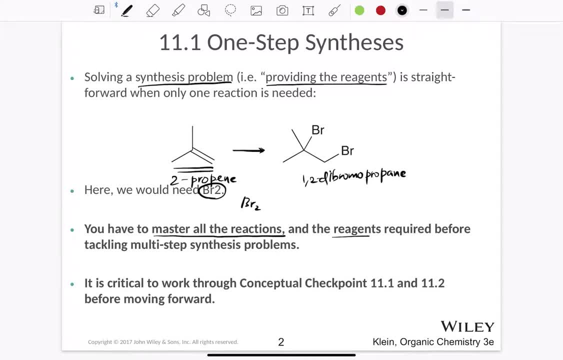 possible in an organic reaction, and we also need to know all the reagents that are required before tackling multi-step synthesis problems. So it is critical to work throughout, Before the work through everything that we discussed before this, before we go through the next parts. 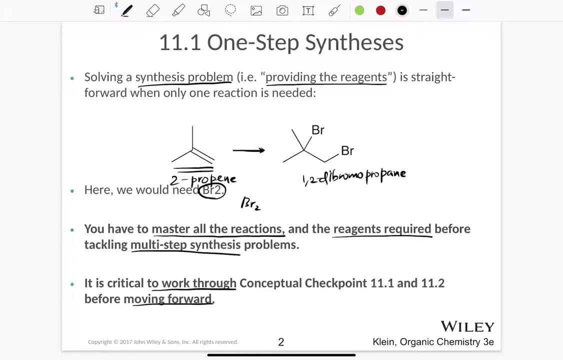 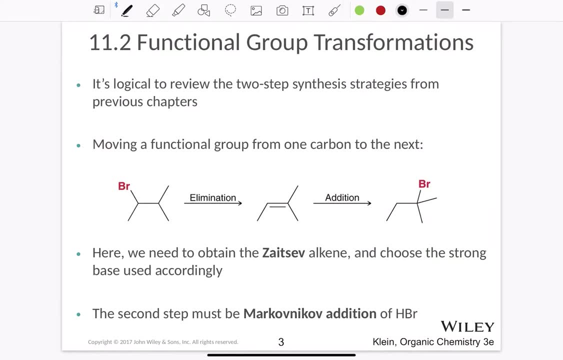 So pause the video right here, go through the summaries of all the chapters before this and try to come back to this chapter Now. so let's talk about the first one, which is functional group transformations. So it is logical to review the two steps in this strategies. So, from the last previous chapters that we discussed, 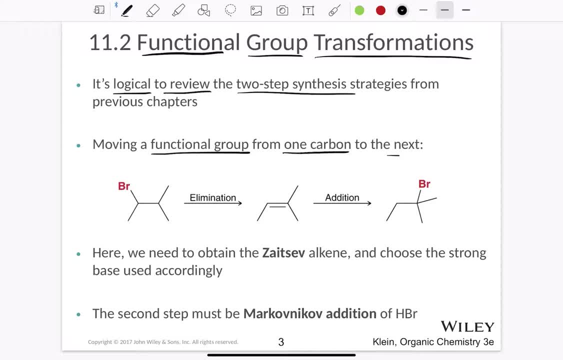 Whenever we are moving a functional group from one carbon to the next. So here the functional group we are choosing is bromine, So the final compound is this one. So I'm moving this bromine from here, this carbon, from this carbon to here. 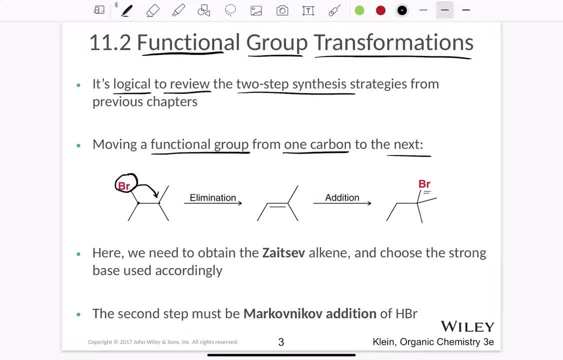 Now this brings up the question: how do I do that? I cannot do it in a one-step process, So the first thing that I'll do is that it undergoes an elimination reaction that eliminates the So that eliminates the bromine. Next I will have to do addition. 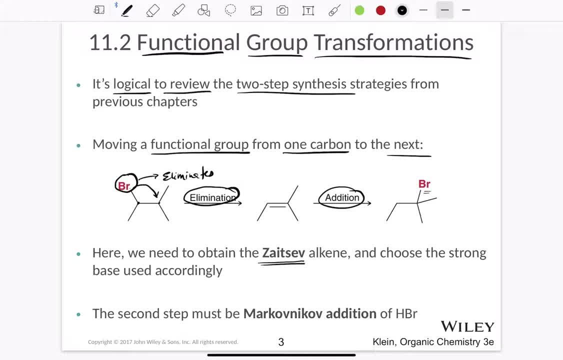 So here we need to obtain a Zaitsev alkene, meaning that we have to obtain a more substituted alkene in the first step. So remember that part Next. so to obtain Zaitsev alkene, we need to choose a strong base. 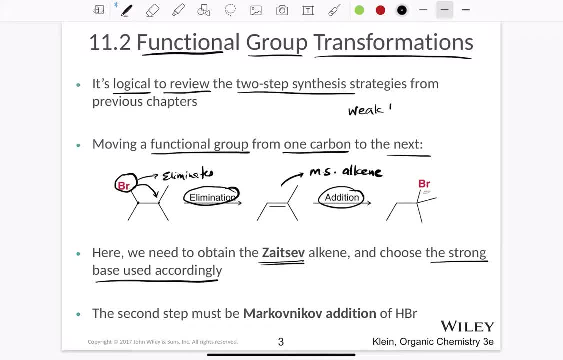 So if you use a weak base, we get a Hoffman product. If we use a strong base, we get a Zaitsev product. So the second step is addition. Here notice that these are the two carbons that are there. 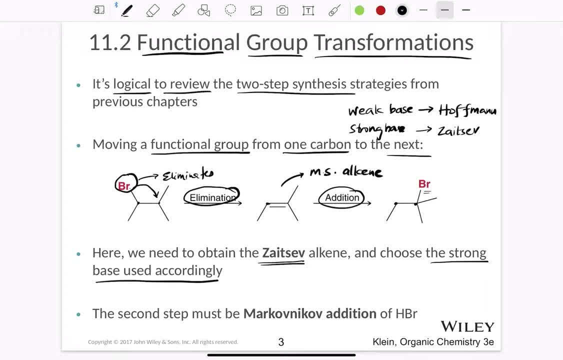 Now the two carbons are being added. so the carbon here is being added with a hydrogen and the carbon here is being added with a bromine. So we know that it's an HBr addition, But we want to know whether it is Markovnikov or Antimarkovnikov. 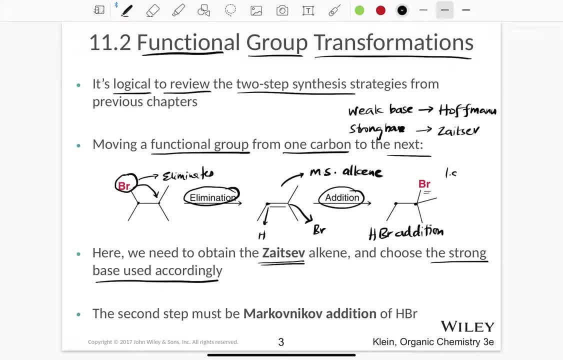 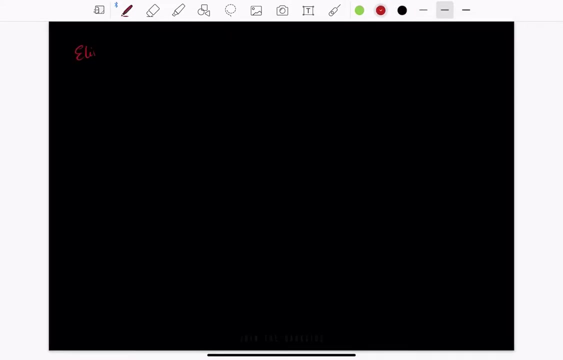 So it says that Markovnikov is that here curios: substituted carbon should get hydrogen, the more substituted carbon should get bromine. so here it matches the sign. so this is Markovnikov addition. so just in this reaction we discussed two main processes. one: we discussed the process. 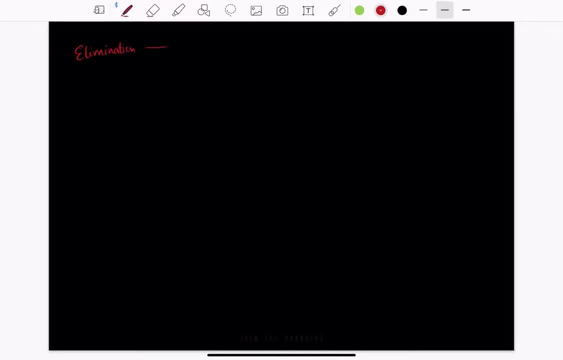 of elimination, especially referring to the Zayasyev elimination. we also discussed addition in this. we discussed hydrobromination, especially in Markovnikov addition. that is why it is important that you review the chapters before this before we come back to this chapter next. 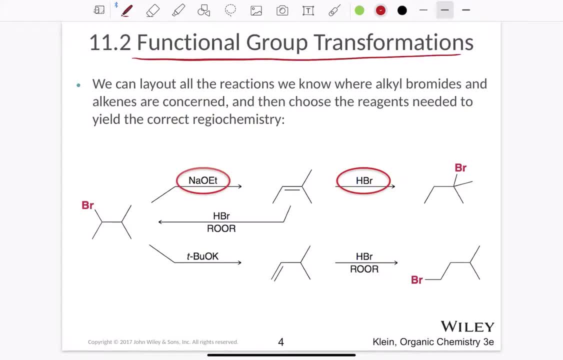 so these functional group transformations. we can lay out all the reactions we know where alkyl bromides and alkenes are concerned and then choose the reagents that are needed to yield the correct regiochemistry. here regiochemistry refers to either Markovnikov or anti-Markovnikov as an 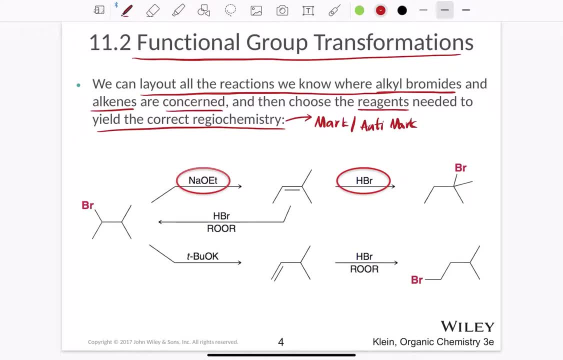 example, or it can also relate to elimination, so it can also refer to whether it's a Cysa product or you get a half mon product. In the first reaction we saw if we use a strong base we get the Zayasyev product, but if you use a weak base, so this is a simple base which is 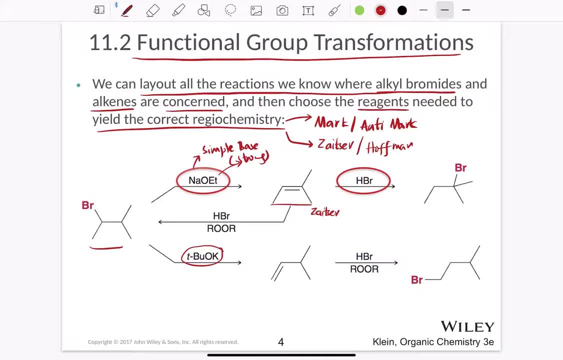 generally a stronger one, so we get a Zayasyev product. here we we use a complex base, a complex base, so we get a Zayasyev product. here we use a complex base, so we get a infrastructure system. here we use a complex base, so we use a complex base. so we get a Zayasyev product. so we project guys. so we project guys, so we present a selection product. so we just see, if anybody now photos of all these components we alreadysoichし. so we get a transobourmanik system. so we transition with the previous procedure. we firstual test, then from that we switch to quark energy management. 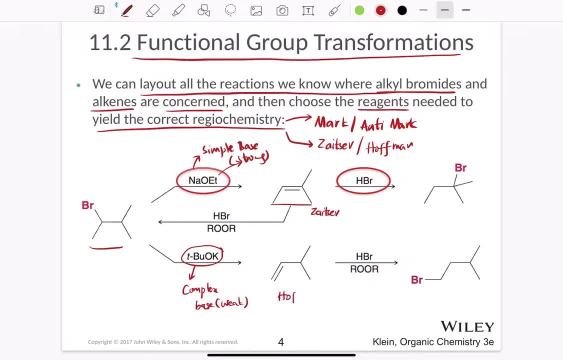 which is generally a weak one, which gives us a half-moon product Now using the ZYSA product. next, if you do HBR addition, there are two ways you can do. One is Markovnikov addition, the other is anti-Markovnikov addition. So Markovnikov addition, there is no peroxides. 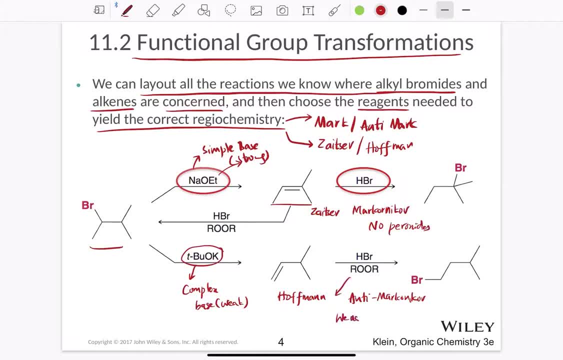 Here we use peroxides. So that's the difference between the two reactions that we just saw. So we can lay out all of this. So if you want to do the back reaction from ZYSA product back to the product, we can use an anti-Markovnikov addition. Notice that you can get back the 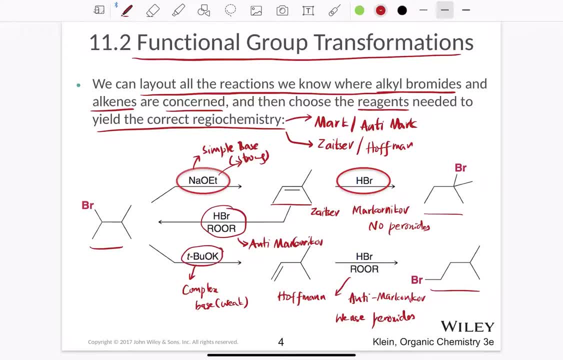 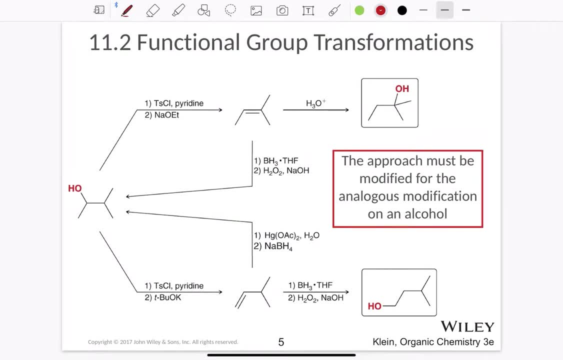 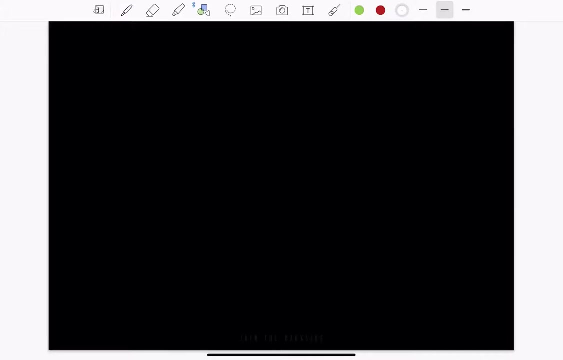 same product back again. So this is one way. The other way is getting back part again. Next, let's say here: if you are using a compound like this, Here we want to transform the functional group from one carbon to the other carbon. So let me write it down separately. 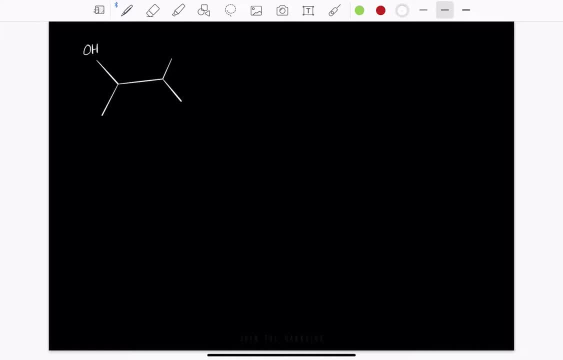 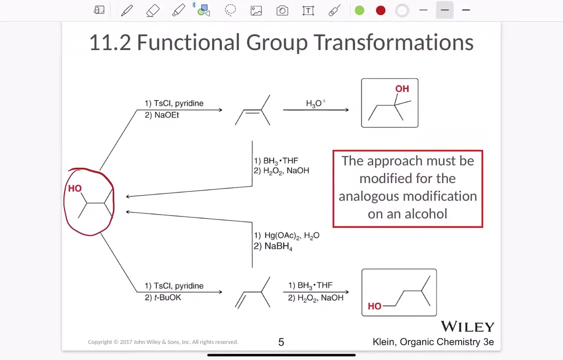 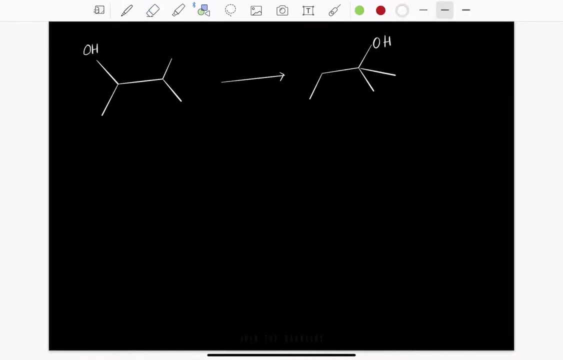 So this is the OH group. Now our idea for the final product is to convert this into this, So we want to move the final product to the other side. So this is the final product that we are looking for. So how do you do this process? 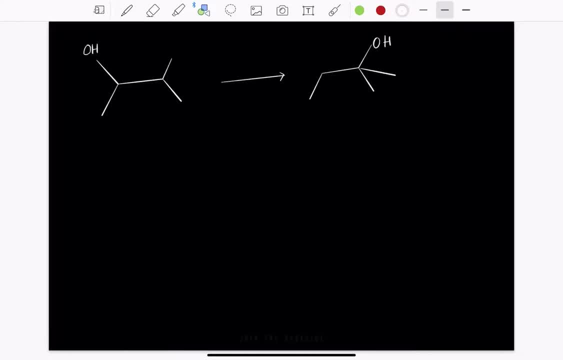 So the first thing to remember is that this test to first undergo OH here is not a good leaving group, So we will have to convert it into an alkyl halide. So the first step here involves converting. 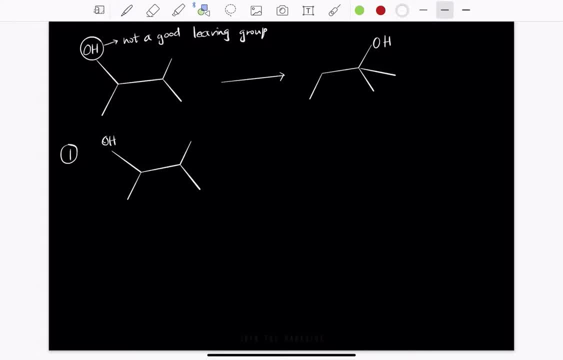 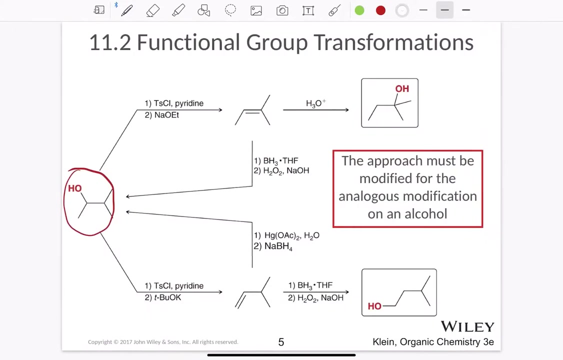 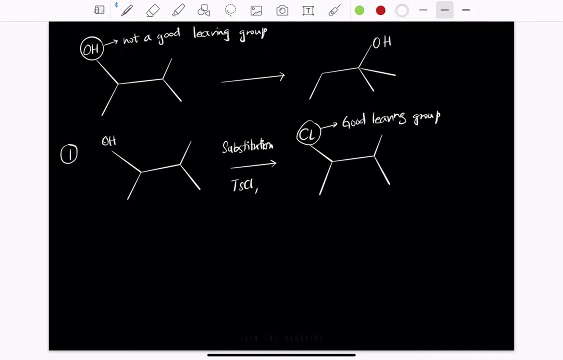 So we are going to use TSCL and Piridine. 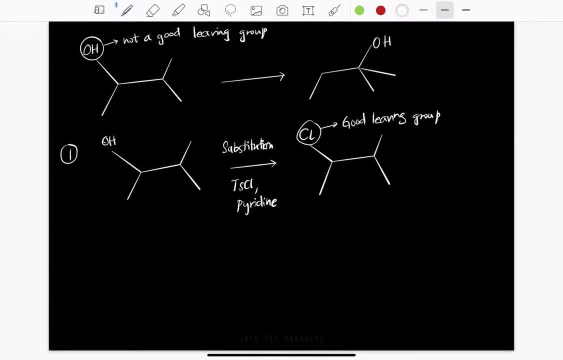 And Piridine. Once we have done this, now The next one is used to This compound, The alkyl halide, And then produce this to form an alkyne. 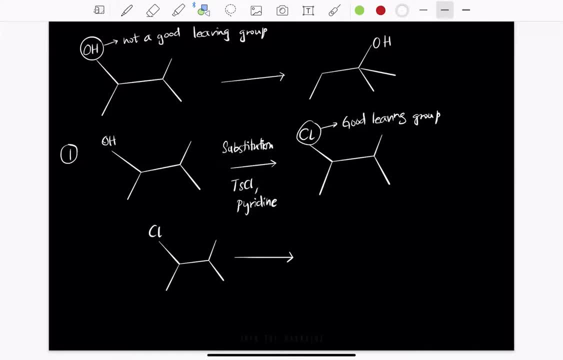 The product would do basically everything. The product would not do anything except start Eigen fluoride and fish oil. so here we are going to need a zysir product, because notice that OH here is on the other side. so we're going to use two. we're going to end up doing elimination next. so in the 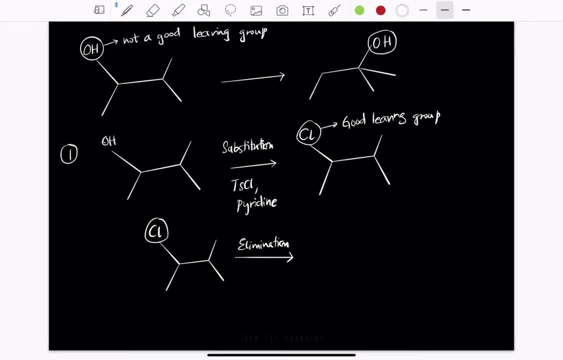 elimination process. you're going to end up with the chlorine moving out and one of the hydrogens going out, so this results in a double bond formation, so you're going to end up with a zysir product. now this elimination requires removal of chlorine, and this elimination is to take place so that 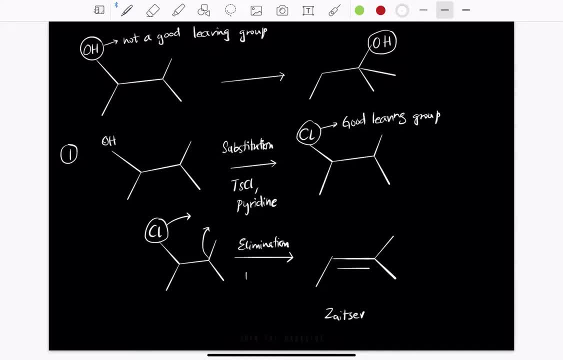 it forms a zysir product, so we need a strong base. so the strong base here we're going to use is NiOeT. so remember that we're going to use a simple base, which means it's a strong base. now, once we get this, we're going to have to put OH on that. so here in the next process, 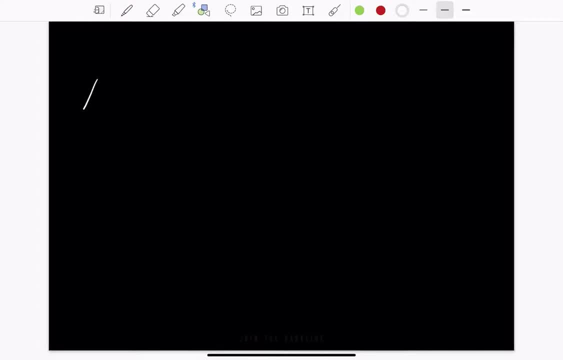 we already have a zysir. we have a zysir alkene. in the next process we're going to have to do addition, but here the final product requires hydrogen and OH being added. so we can think about the process here as the process of acid catalyzed hydration. 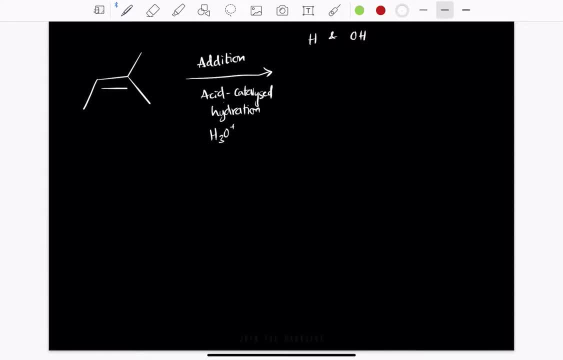 so, which means here we're going to use H3O plus, right? so we're going to end up with H3O plus. now the final product will be OH. so this is how you get the final product. So this is how you get the final product. 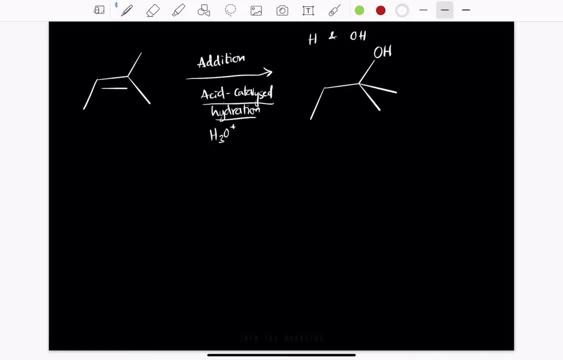 So here notice that acid catalyzed dehydration, hydration results in Markovnikov addition of hydrogen and OH. so which means that here there are two carbons. this is one carbon. there's the second carbon. this is the less substituted carbon, this is the more substituted. 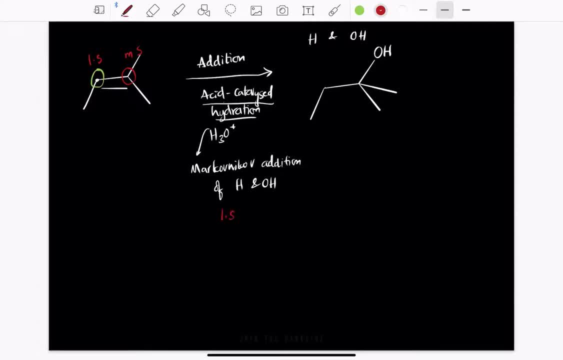 carbon. so the idea of Markovnikov addition is that the less carbon, less substituted gets hydrogen and the more substituted gets OH. so this is the synthesis reaction. now you can summarize the full compound like this. so here in this process we have reagents. number one is TSCR and pyradine, number two is elimination. 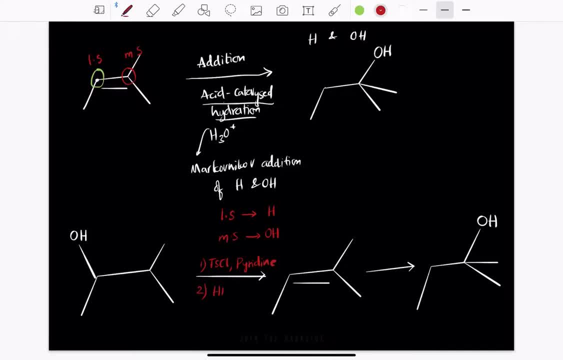 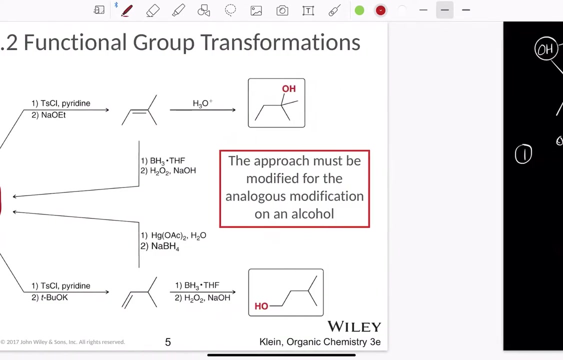 So here elimination occurs with HBr. So elimination occurs with a weak base. we use NOoEt in the second process. the next process, we have H3O plus and H2O. So that's your final reaction. So the approach refers to Where we are looking at and what are we going forward to. so this is the process that we are looking at. 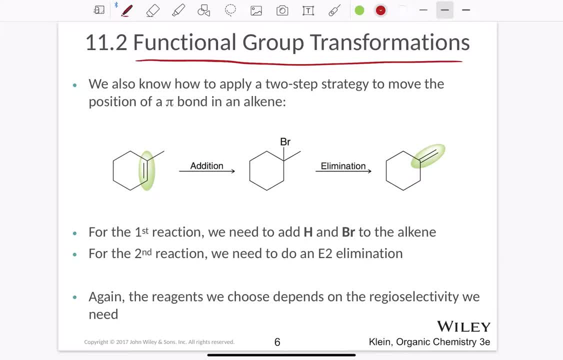 Now, Functional group transformations can also take other methods. So we can also use a two-step strategy to move from a position of a pi bond into an alkene, So where we are moving a pi bond here. So here Is the motion of a Pi bond. so the pi bond is right here. We want to move it to the carbons, these two carbons. 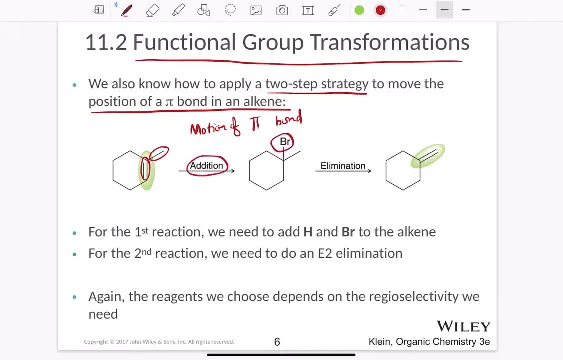 So the first thing I'm going to do is addition reaction, which results in the bromine getting added to the more substituted carbon and hydrogen. So Bromine gets added here, the less substituted carbon gets hydrogen. So the next one is elimination. when you eliminate here, this results in the double bond formation on the other side. 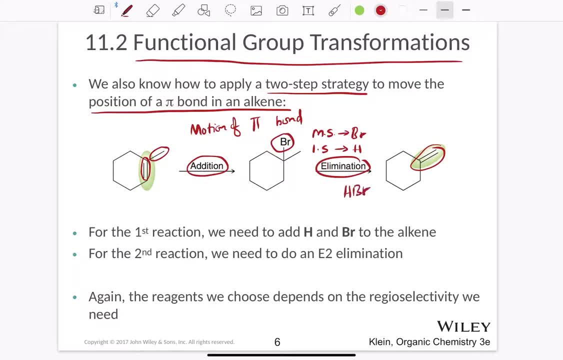 So where the HBr gets eliminated. So the first reaction we need a hydrogen and bromine to the chlorine and the second reaction we do an E2 elimination. so Reagents that we choose depends on the region selectivity that we need. So remember that the region selectivity is the main point that we are looking at when you have synthesis reactions. 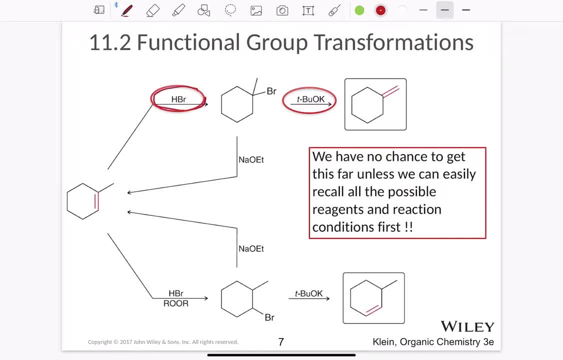 Now. so in this reaction, the first one is HBr, The reagent is HBr, So hydrogen and bromine get added to the compound. So here there's hydrogen and here there's bromine. Next, because we are looking at elimination reaction and the double bond, 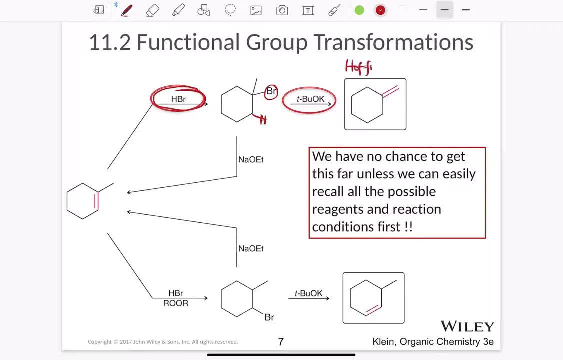 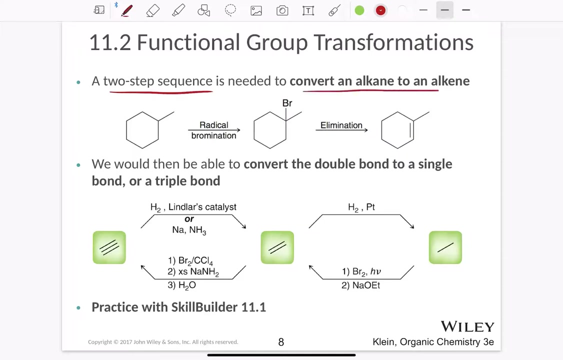 So we want a Hoffmann product. So we want a Hoffmann product. so, which means that we're going to end up having to use up a complex alkyl Complex base. Now this is the state, the synthesis of the reaction in itself, So a two-step sequence is needed to convert an alkane into an alkene. 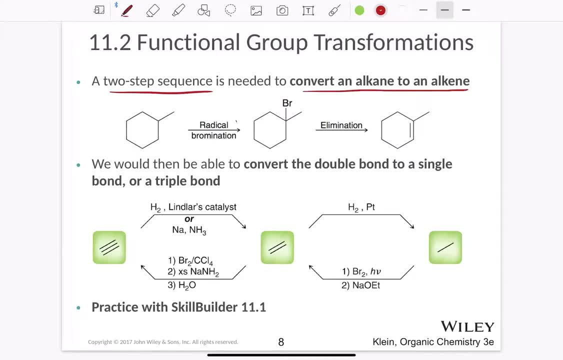 So when you want to call for an arcane. So the first thing that we do here is radical permutation, where we add bromine. The next step is elimination. that results in a double bond formation. Here we are looking at Zeiss product, So which means that here elimination occurs in, as I say, product. so we're going to end up using a simple alkyl. 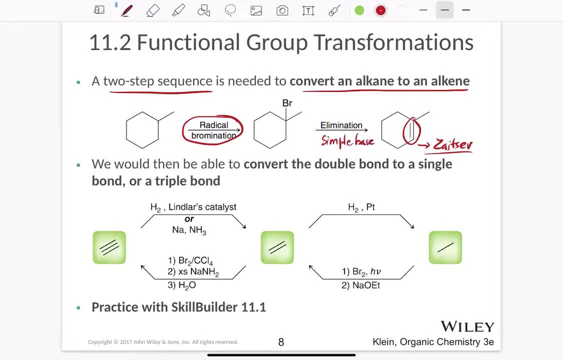 Simple base. So we're going to end up using, for example, Next we'll be able to convert a double bond to a single bond also, or to a triple bond, for example, poison catalyst such as Lindar. For example, poison catalyst such as Lindar, Lindar's calendar's catalyst- can be used to produce a triple bond to a double bond. if you want to further continue the reaction, we can use. 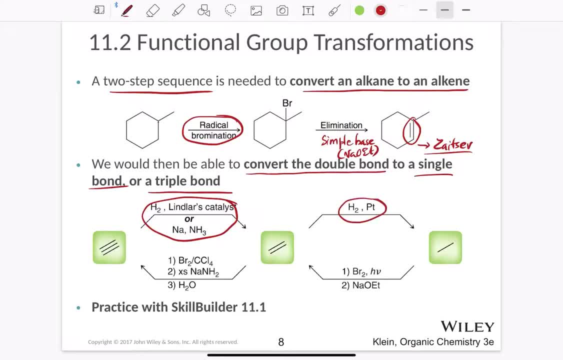 hydrogen, so catalytic hydrogenation to produce a double bond to a single bond. next, elimination results in the alkene formation right and presence of bromine and carbon tetrachloride and excess sodium amide causes it to form a triple bond. so these are functional group. 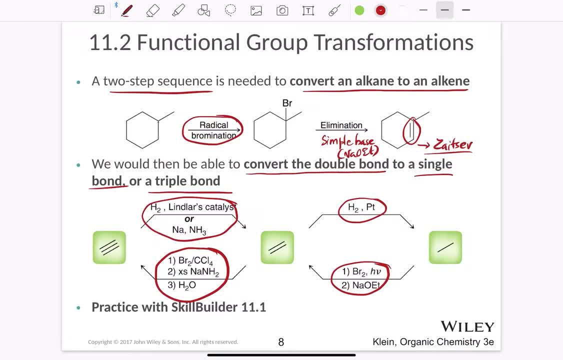 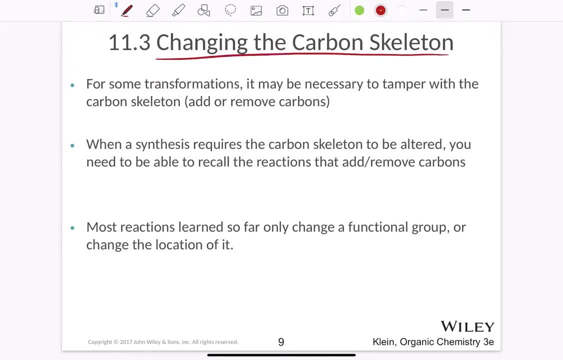 transformation. so this is basically the summary of all the reactions that we saw before in alkanes, alkenes and alkynes. next, changing the carbon skeleton. for some transformations we might need to necessarily tamper with the carbon skeleton itself, which means that we might have to add or remove the carbons. 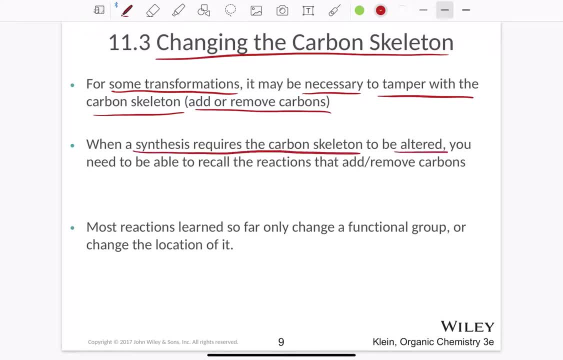 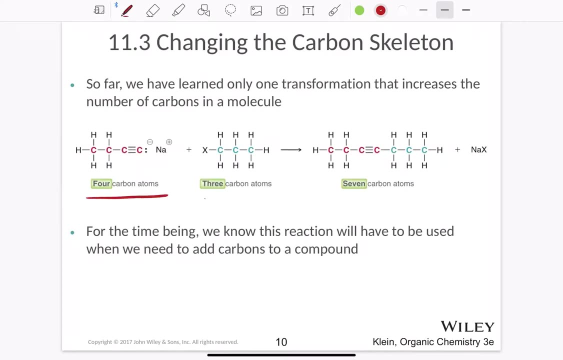 so when a synthesis requires the carbon skeleton to be altered. so you need to able to recall the reactions that add or remove the carbons. so most of the reactions learned so far only change a functional group or the change in the location of it. so for example, here if you have 4-carbon structure and a 3, 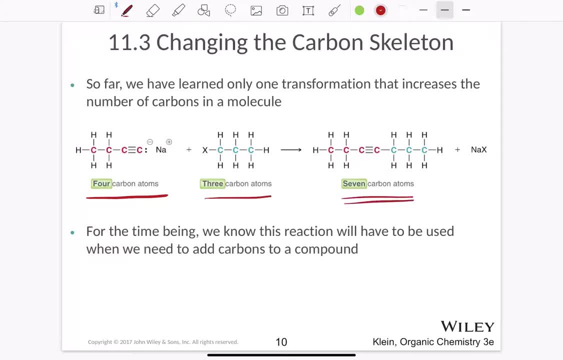 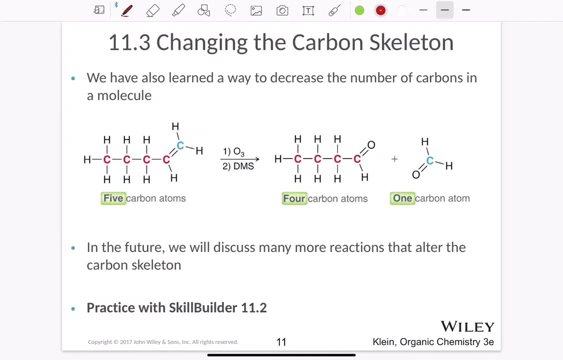 carbon structure, we might need to form a 7 carbon structure. so we only have learned only one transformation that increases the number of carbons in a molecule. so for the time being now we know that this reaction will not be used. we'll use that to add carbons. So one of the main reactions that we change the 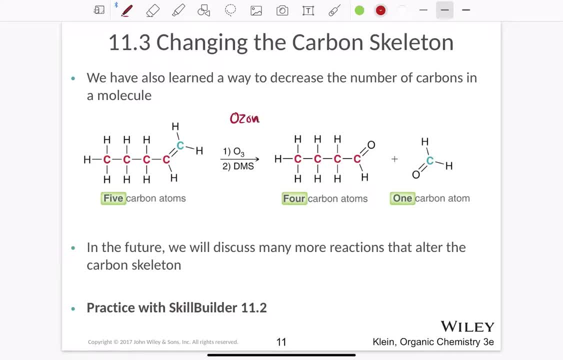 outer of the carbon structure is the process of ozonolosis. Ozonolosis is additionally adding ozone and dimethyl sulfide where it splits the alkane alkene. So here it splits the double bond and forms oxides. So oxides can be. 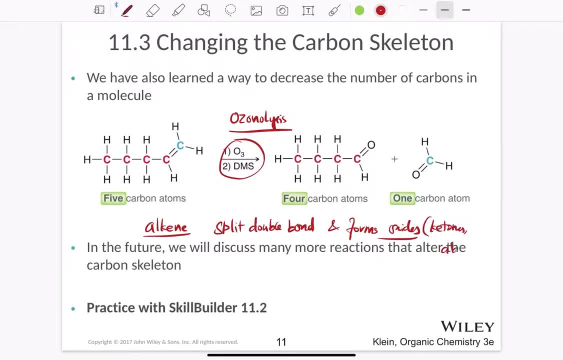 ketones oxides can be aldehydes. So, depending on the structure it can have, the most common structure form is a double bond O and whatever is the side chain form that results in its proportional oxide. So that's it, Thank you. 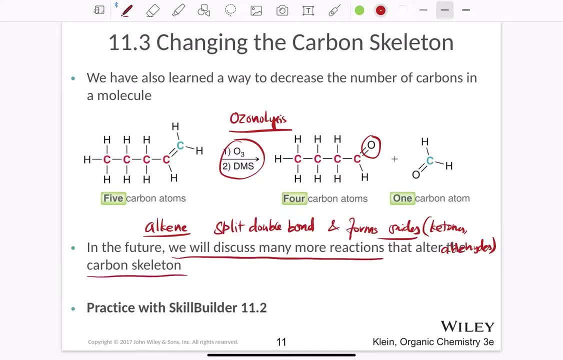 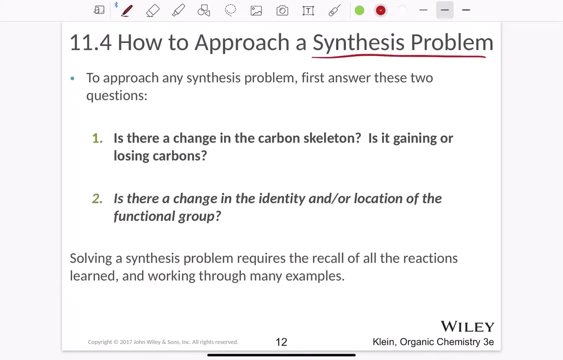 So in this we will discuss many more reactions that can help. in the future we'll discuss many more reactions, but for now remember ozonolosis is our main process to split or change the outer of the organ structure. Now, how to approach a synthesis problem. So to approach any synthesis problem, first answer main. 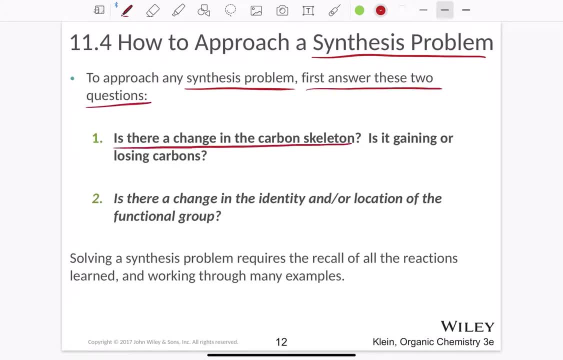 questions. two main questions. One: is there a change in the carbon skeleton and is it gaining or losing carbons? So second, is there a change in the identity or the location of the functional group? So solving a synthesis problem requires the recall of all the reactions learned and working through many examples. So the 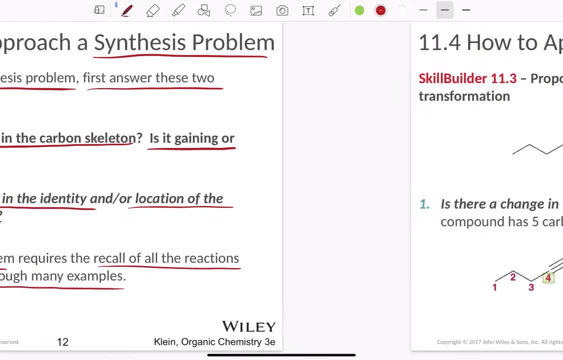 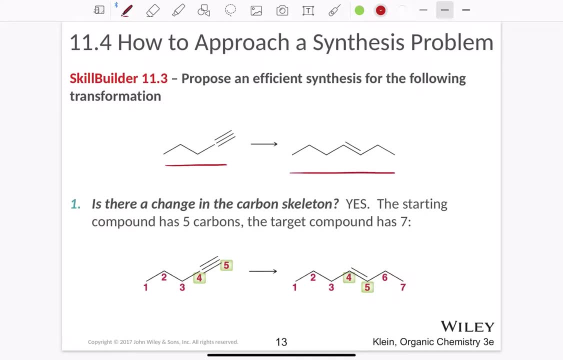 more you work through examples, the more it is easier to understand synthesis problems, For example. here they have given us a problem where they have asked us to convert this into this structure. So let me copy it, So, let me copy it, So, let me copy it. 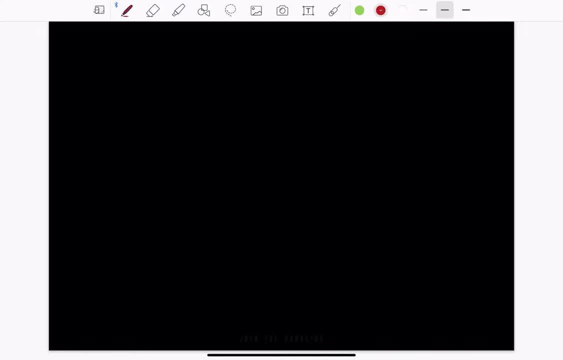 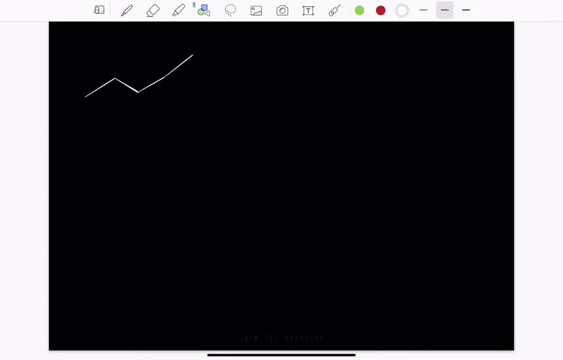 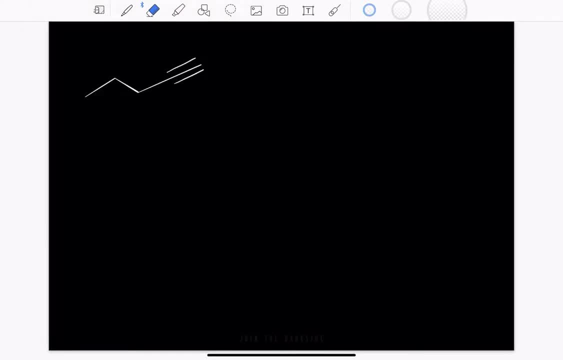 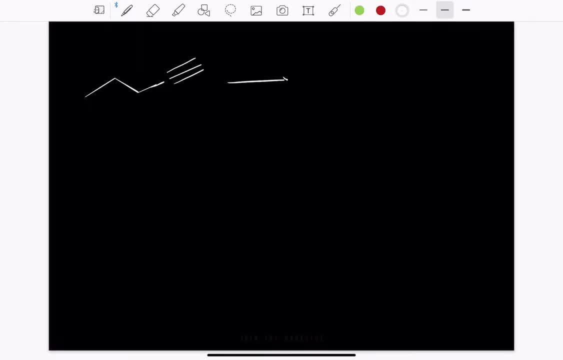 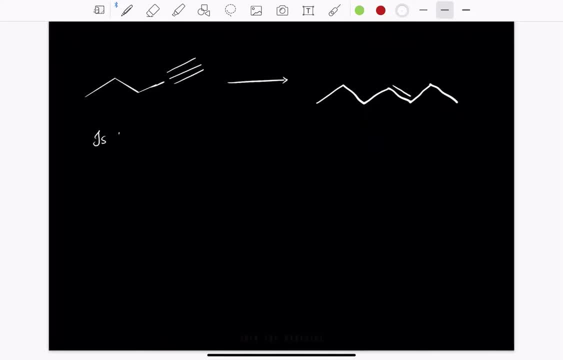 The first step: is there any change in the carbon skeletal? So first remember: is there any change in the carbon skeletal? So here we can say yes, because notice that here you have 1,, 2,, 3,, 4,, 5, and here you have 1,, 2,, 3,, 4,, 5,, 6,, 7.. 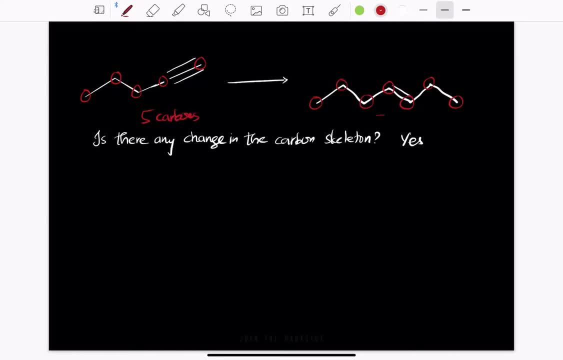 So here you are, converting from 5 carbons to 7 carbons. Next second question is: is it gaining or losing electrons? Sorry, losing carbons. Here we can say: yes, it is gaining carbons. So we have answered the first two questions. 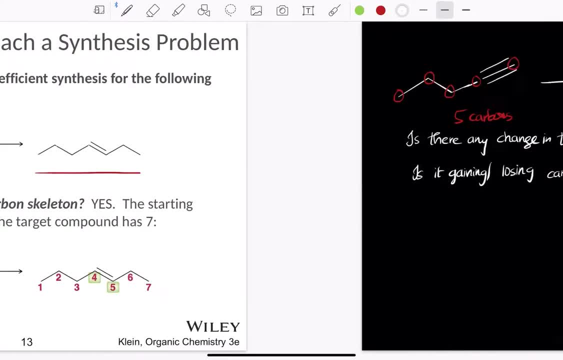 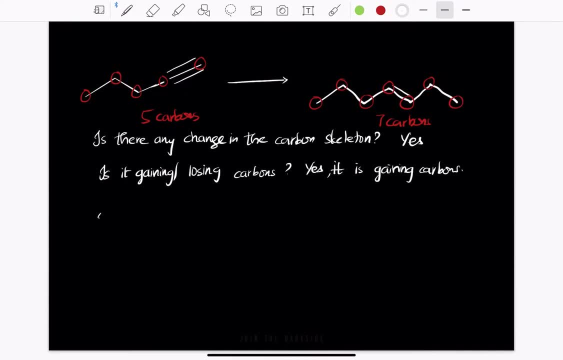 So it is still going to gain carbons. So we are starting compound with 5 carbons and we are ending with a compound of 7 carbons. Second is: is there any structural change? Basically meaning that is there any identity change? 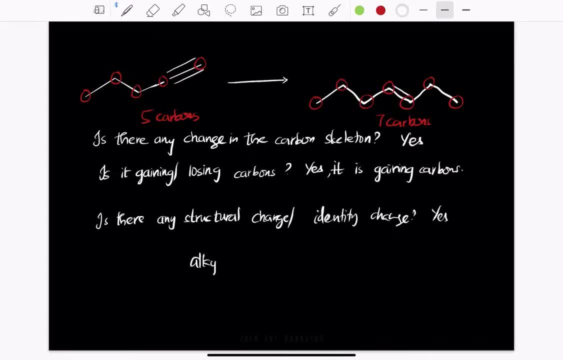 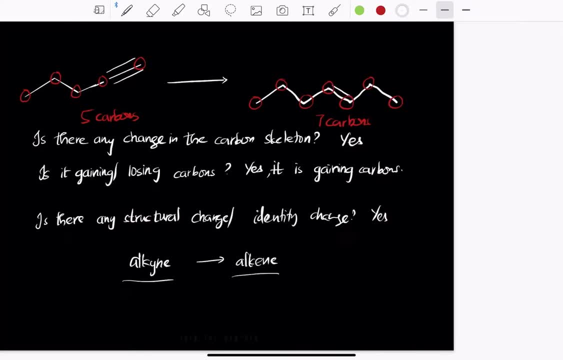 Here we can say: yes, So we are converting an alkyne into an alkene. So we are converting an alkyne into an alkene because notice that here we have a triple bond and we are converting it into a double bonded carbon. 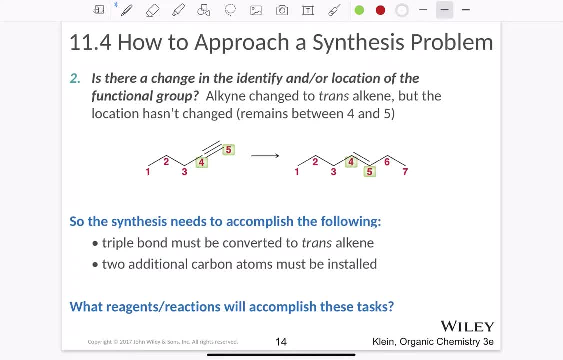 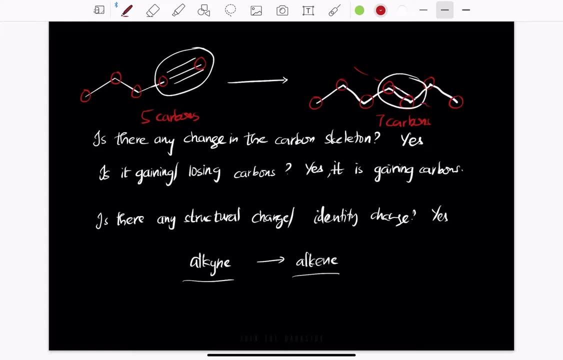 So to synthesis, we need to accomplish the following process. One, we have to convert the triple bond into a transalkyne. Second, we need to convert, we need to add the two additional carbons that must be installed. So here, notice that in this structure, if you flip this structure, it's a, there is a structural change and is there a change in the radio selectivity. 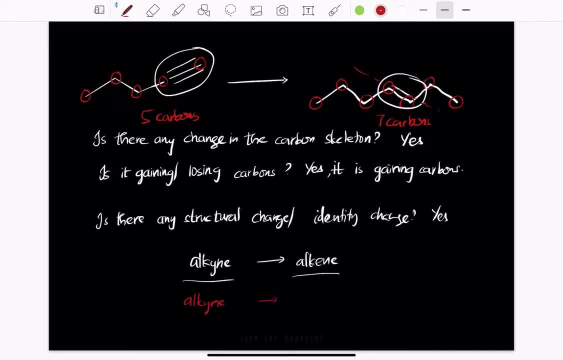 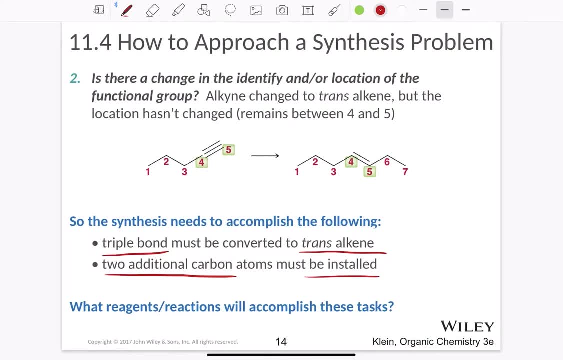 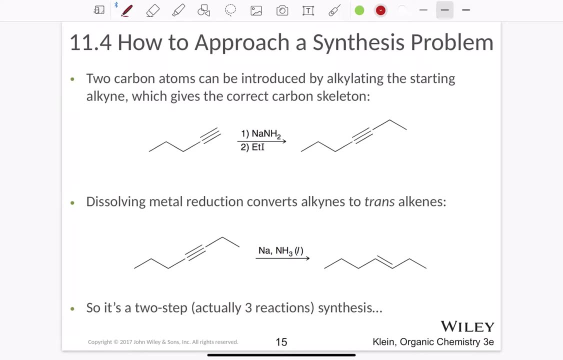 Here we are converting an alkyne into, specifically, a transalkyne. So we will focus on three, these two steps. So what are the reagents that need that we need to accomplish these tasks? Number one: We know that to convert a triple bond into 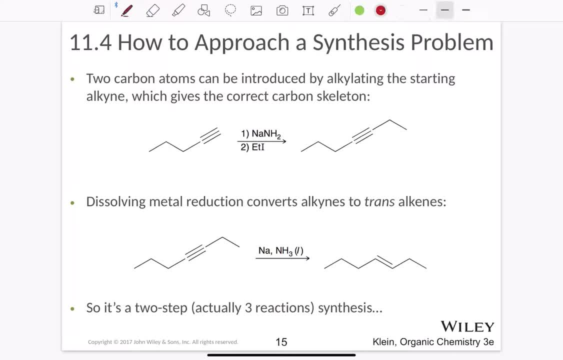 So we need to first convert, We need to add the number of carbons, We need to add carbons, Adding carbons. the only process that we know is to convert a terminal alkyne into into an internal alkyne. so the first thing is we are going to use sodium amide and ethyl iodide. 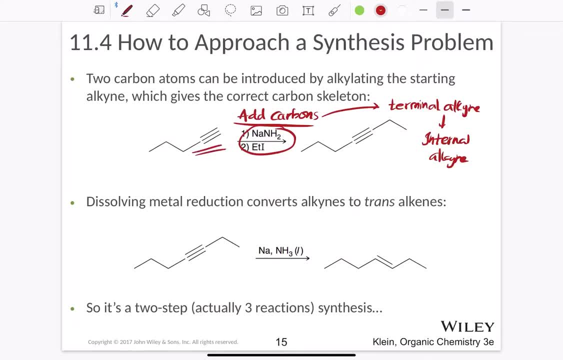 and we are going to convert a terminal carb, terminal alkyne into an internal alkyne. notice that here ch3, ch2i, this is the part that is being added to the triple bond, next dissolving it, metal reduction so converts it from alkynes to transalkyne. so this process, in the presence of 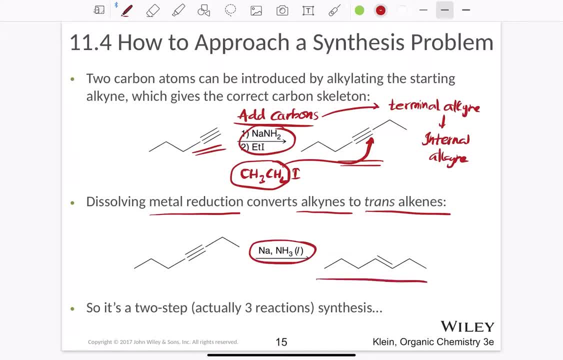 sodium and nh3 results in an alkyne formation. so where we are going to convert from an alkyne into an alkene, specifically a transalkyne. so here it's a two-step process. so in sense it's a three-step process. but you know, we can consider. 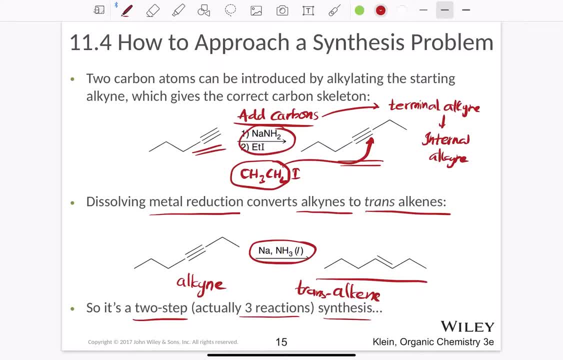 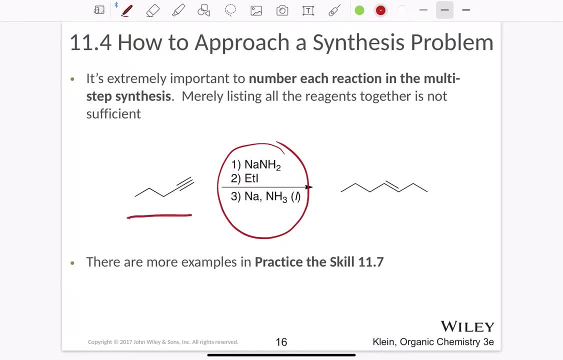 it to be a two-step process because we're only using two steps to convert into final product. so these are the three reactions involved in converting an alkyne into an alkene, a trans alkene. so it is extremely important that we number the each reaction in the multi-step synthesis. 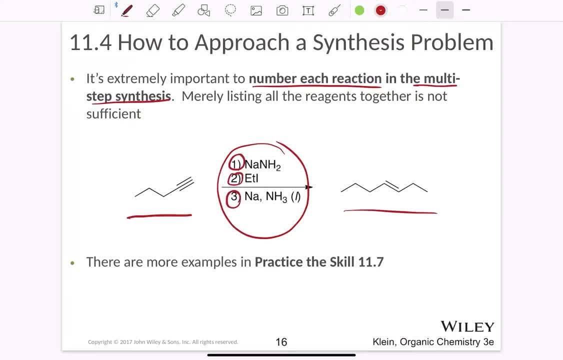 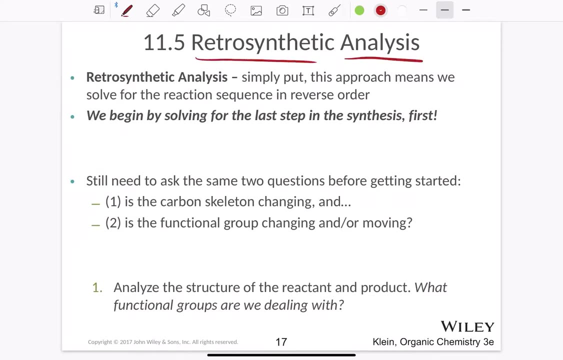 because one, two, three refers to the sequence in which the reactions occur, so merely listing all the reagents together is not sufficient. next, let's talk about another type of analysis, called retrosynthetic analysis. so the name itself says retrosynthetic, which means that this approach 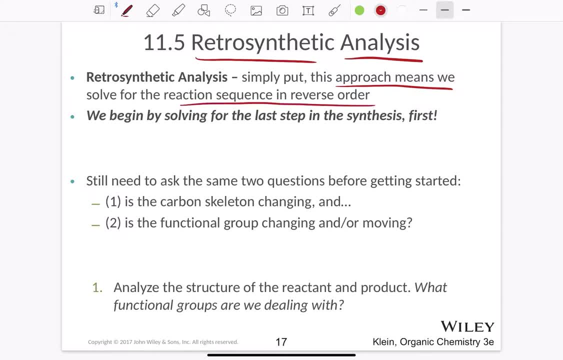 we solve from the reaction in the reverse order. so we begin by solving the last step in the synthesis first, and then coming back to the backward step. so whenever you see this word retro, it means backward. so whenever you're retrofitting something, it means that you're working backward. or to see: 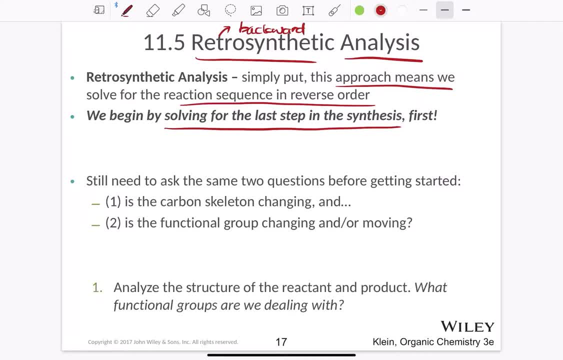 a series of reactions combination and you're going to work back in the same way. you have to, whether how it has originally started. now again here also, we need to ask the same two questions: is the change? is there a change in the carbon skeleton or is there a change in the functional? 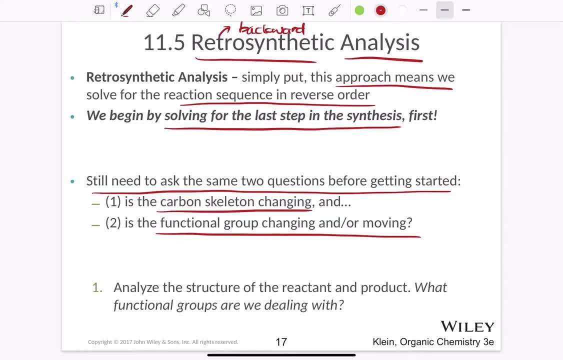 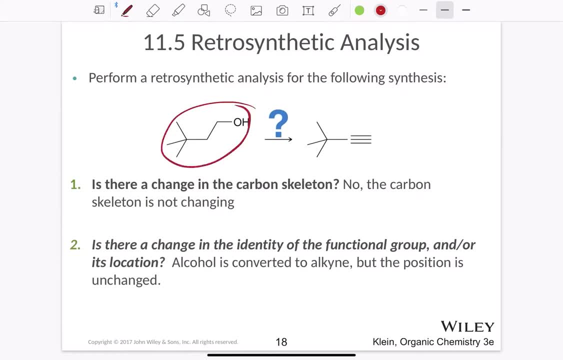 group, changing or moving. next first step is to analyze the structure of the reactant and product and what are the functional groups that we are dealing with? for example, here in this compound we have oh group, so that has changed to a triple bond. so we have an oh group converting into a triple bond. so the first step that we know is: let's start. 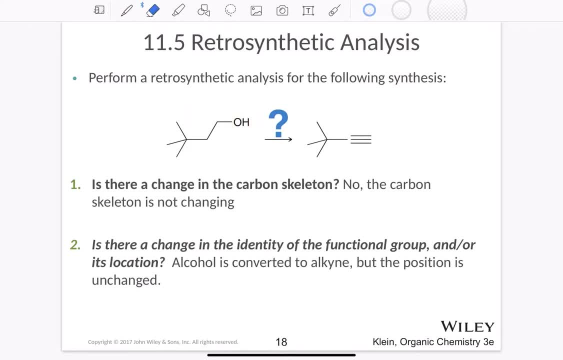 with the first step, which is: is there any change in the carbon skeleton? let's check the number of carbons. so number one, two, three, four, five, six. one, two, three, four, five, six. so here also there's six carbons. here also there's six carbons. so there is no change in the number of scale carbon skeletons. 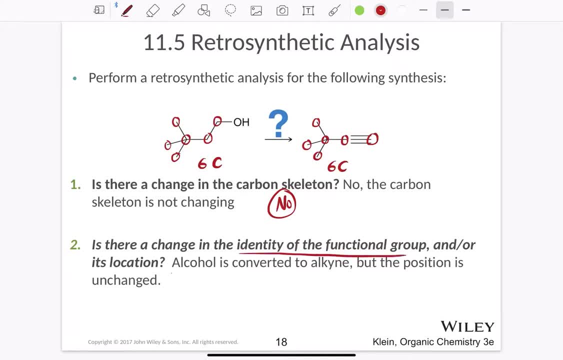 next, is there a change in the identity? yes, because we are converting an alcohol into an alkyne, but the note is that the position is not changed. so wherever the alcohol was attached, there itself is the triple bond. so remember that concept. now, what are the reactions that we need to convert? 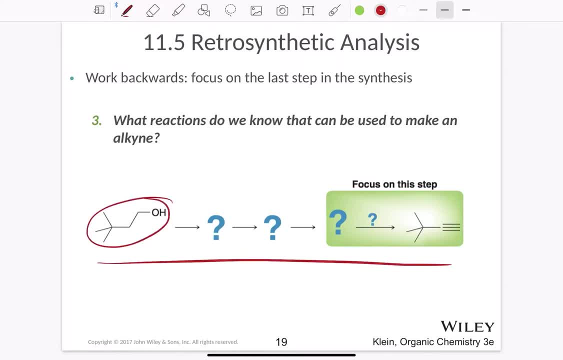 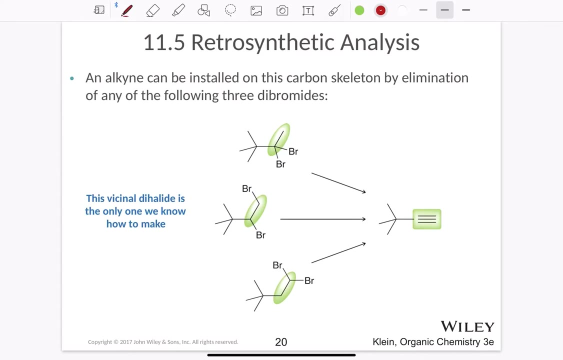 the process from an alcohol to an alkyne. the first step is to look at the last step of the process. so the last step involves looking at the last five. we do not know the byproducts in the middle, but we want to focus on mainly the last step. the last step results in converting the alkyne. 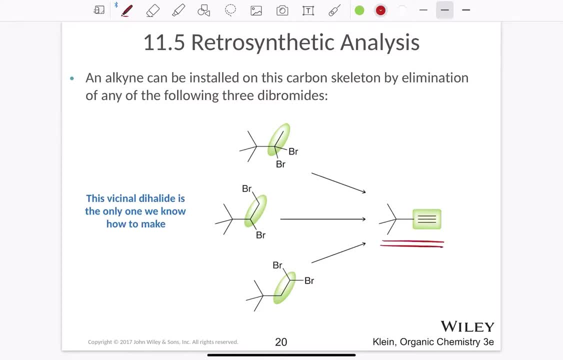 so we are going to convert the alkyne into some sort of an, an alkyne with a substituted alkyne, because for it to bond with an oh group it needs to have something there. in that point. now the vicinal dihalite is the. 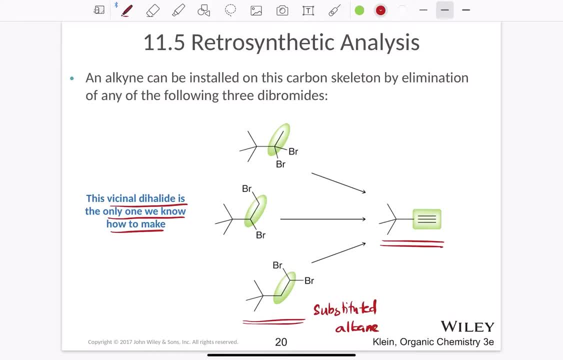 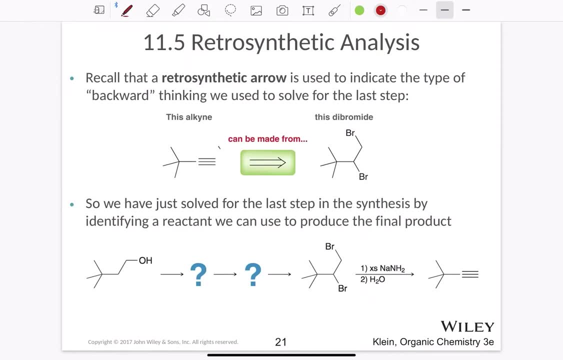 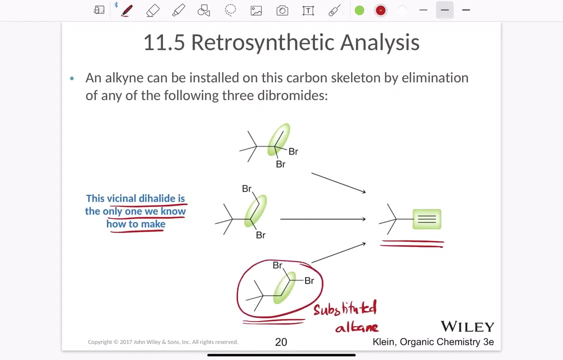 only one that we know how to make. so, because this is the only way that we can make that process, so we can use that to start the process. so the first thing we can do is we can take this alkyne and we want to convert it into a vicinal dihalite notice that we do not know how to use. convert this. 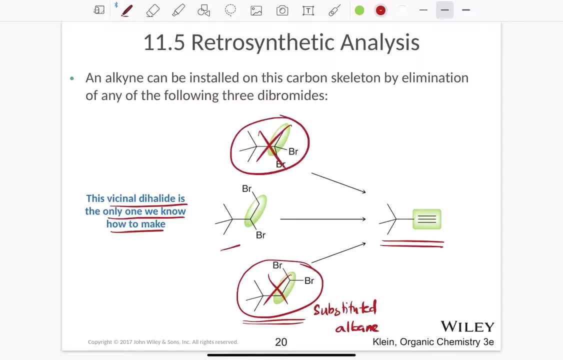 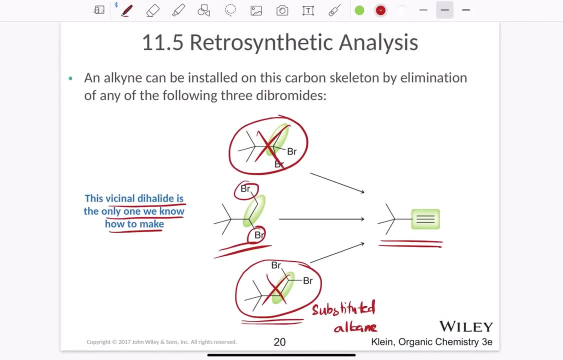 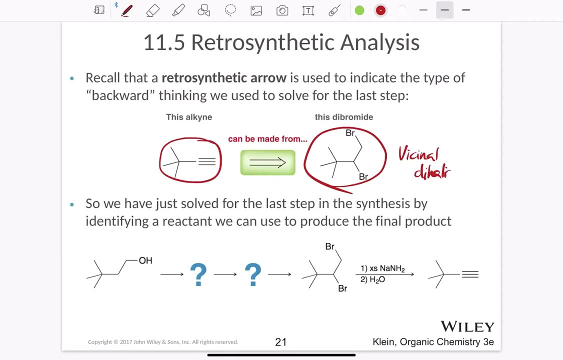 and we do not know how this reaction works. so this is the only thing that we know, where we have two carbons, two alkynes that are attached to the same card, to the adjacent carbons. so that is the vicinal dihalite next. so we know that the reagent that is used is excess sodium amide and water. so the first step is: 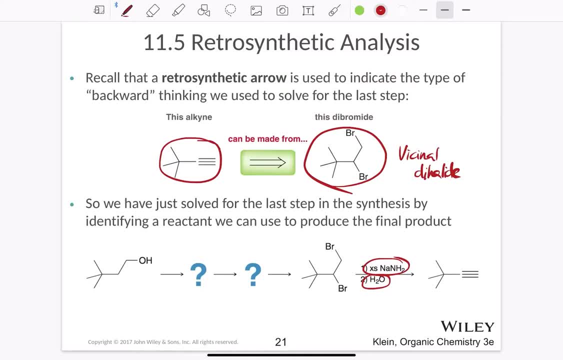 excess sodium amide, converts it from an alkyne into an alkene and then adding water convocates adds it undergoes acid catalyze hydration now. so we know that we are converting this into bromine, so we are adding two bromines here. 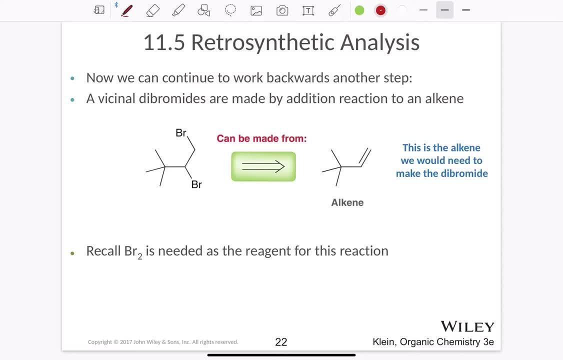 the next process is: we can continue backwards again, so we can use this and if it undergoes elimination, it can form an alkene. so which means that here we are going to add a dibromide to alkene. so from adding br2 to alkene produces dibromide. now we know that this process works. 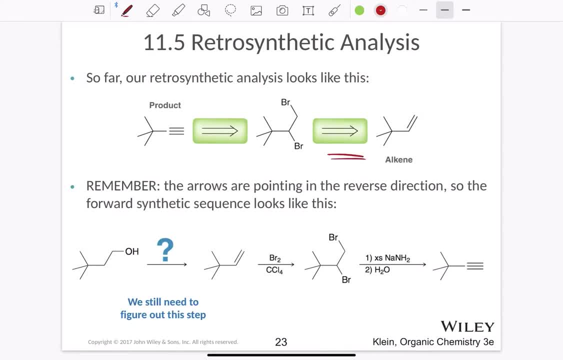 so the second process is also done, where we are going to use dibromide, so in presence of ccl4. so, and the presence of ccl4. now we know that this is the alkene that we have used. now we know that there is only one step to figure out, because we already know all the steps. 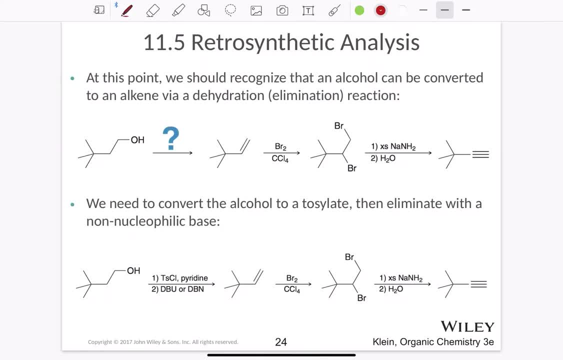 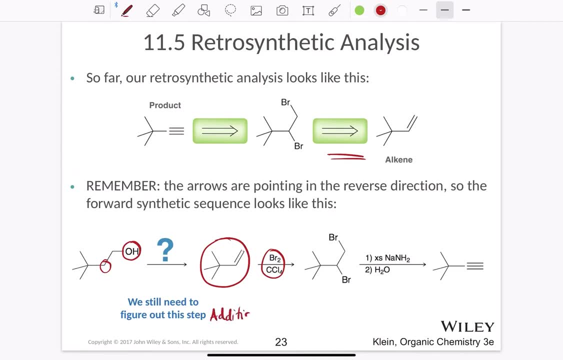 notice that this is the less substituted carbon. this is the more substituted carbon. now what? what reaction is there here that can does that? so the here? we know that this is an addition reaction, but here the addition reaction involves h, and oh means that H is being added to the more substituted carbon and OH is being added to the less substituted. 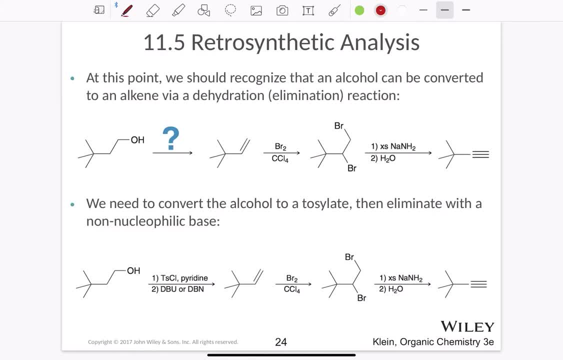 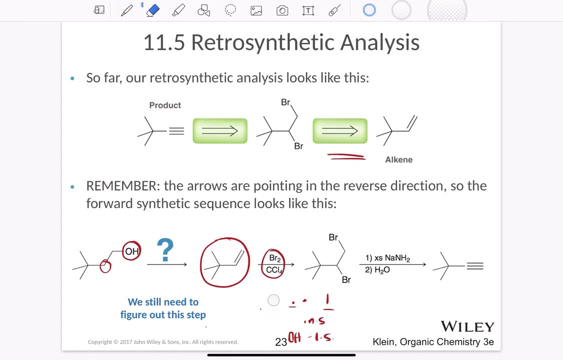 carbon. so here this refers to the first step again, which is: we cannot remove, we cannot add OH directly, we cannot remove OH directly to form an alkene. so notice that this reaction, if you look at the forward reaction, its elimination, if you look at it in the 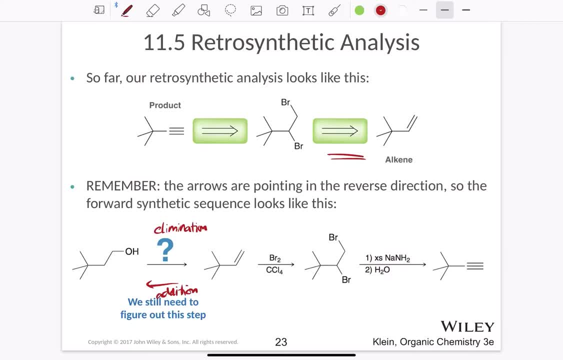 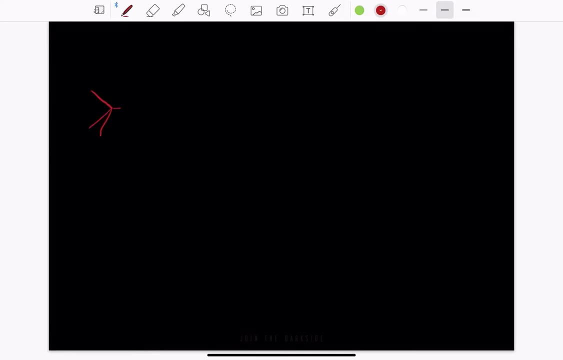 reverse its addition. now we want to know how to do this part of the reaction only. we are looking at how to do this part of the reaction only now. if you look at that part of the reaction, only this part of the reaction only. we want to know how to do that part of the. 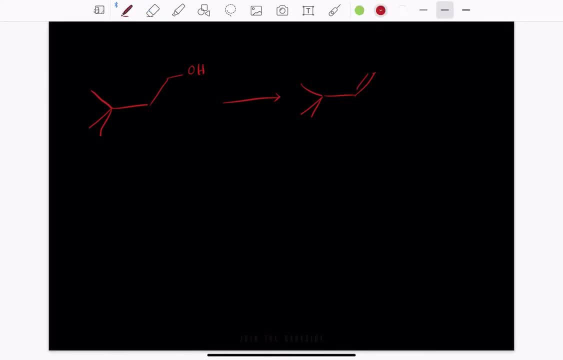 reaction only. so this: we know that it's an elimination reaction, but the problem is in elimination. you notice that OH is not a good leaving group, which means that is a first step. that involves removing OH. imagine of something else. so this process involves first using TSEL and pyrimidine to make it into chlorene. 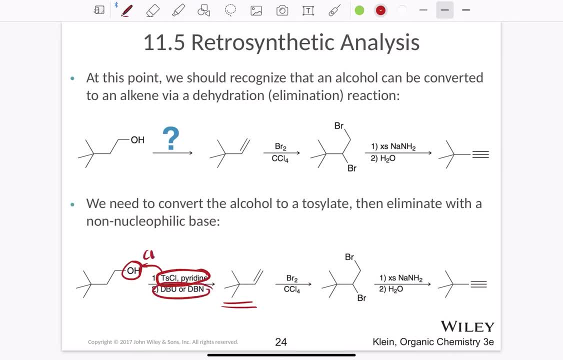 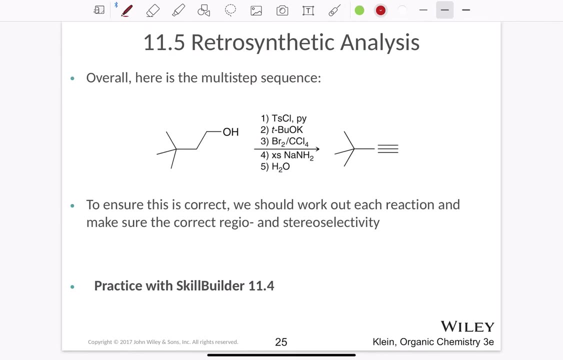 first and then using DD or DBM to undergo elimination reactions. E Всё to reaction. so first step is substitution, the second step is it eliminationあと. So these are the steps that are involved and these are the five steps that are involved in the multi-step process. 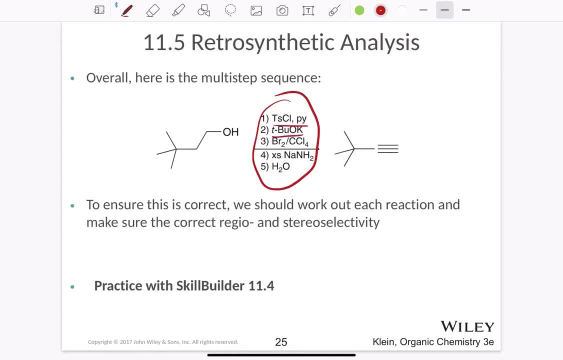 But remember that every step that we know- we have already gone through this multiple times, but we have gone through them separately. now we are using them to work it out collectively in one simple sequence. To ensure this is correct, we should work out each reaction and make sure we have the 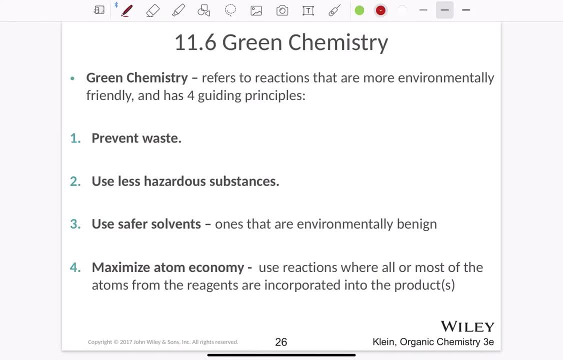 correct regio and stereoselectivity. So next let us talk about green chemistry. So green chemistry refers to the reactions that are more environmentally friendly and four guiding principles. So here we are looking at to prevent waste and we are trying to use less hazardous substances. 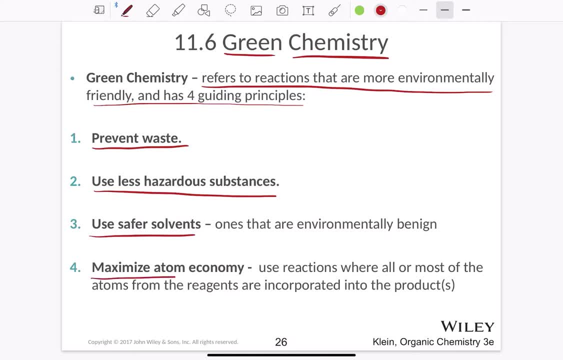 and three, we are trying to use safer solids, and four, we are trying to maximize the atom economy. So one and two are much easier. so we want to prevent waste and use less hazardous substances. Number three refers to only that are environmentally benign where they do not affect energy. 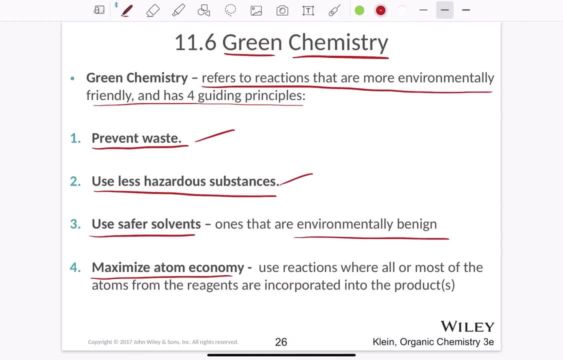 environmental compounds. Number four is maximizing atom economy is to use reactions where all or most of the atoms from the reagents are incorporated into the products. So let us take a simple example of two processes: oxymercuration, demercuration and acid-acid. 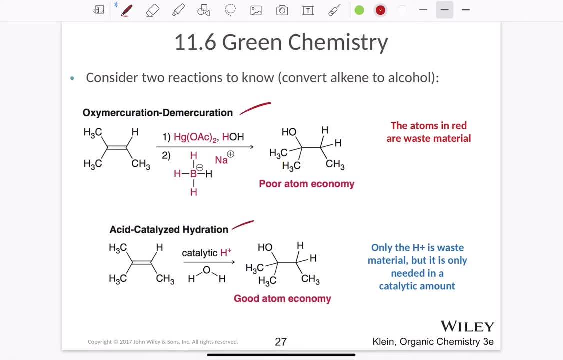 catalyzed hydration. So we know that oxymercuration and demercuration- everything that you see in red- is a byproduct. So the atoms in the red here are the waste material, so which means that this results in a poor atom economy. 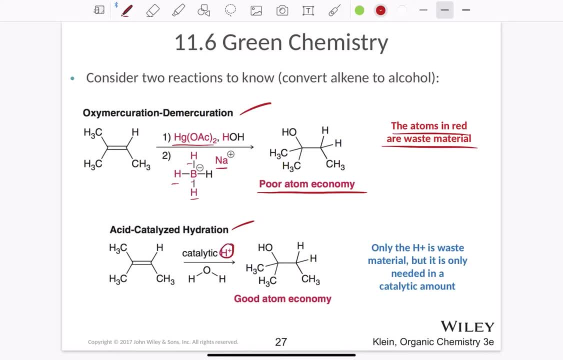 Where there are too much waste materials. Here, the only byproduct is H plus. so because only H plus is the byproduct, we can get this back into the reaction and let it continue into a catalytic amount, so we do not need to use this every single time, more and more so, which means that this has good atom economy. 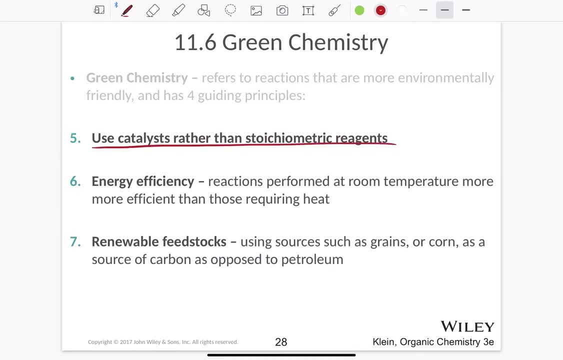 Next, the fifth step is to use catalyst rather than stoichiometric reagents. Number six is energy efficiency, where reactions are performed at room temperature more and more efficiently, And those requiring heat. And number seven is renewable feedstocks, meaning that we are trying to use sources. 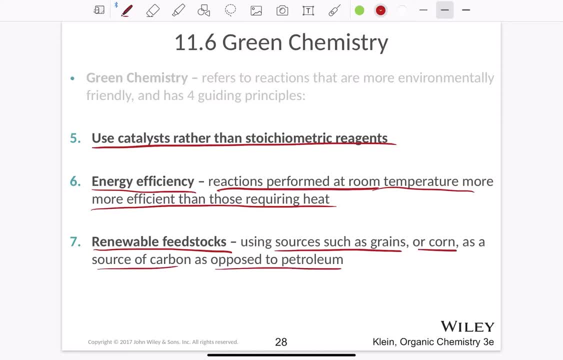 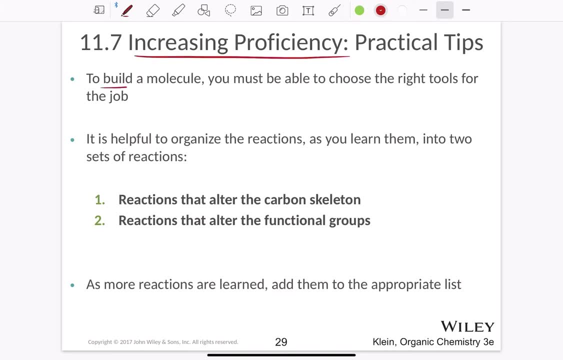 such as grain or corn, as a source of carbon as opposed to petroleum, So increasing the proficiency, the practical tips that we can use to build a molecule. you must be able to choose the right tools for the job, So it is helpful to organize the reactions, as you learn them, into two separate sets. 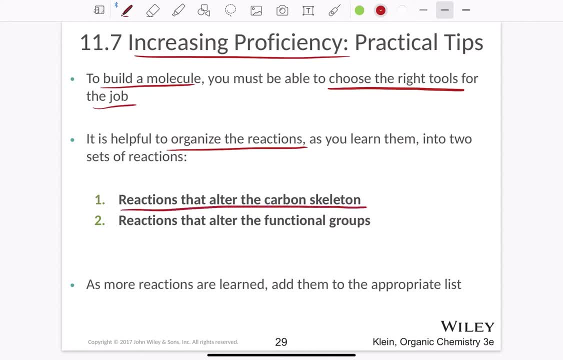 One is the set of reactions that can alter the carbon skeleton, for example reactions like ozonolosis. Reactions that alter the functional groups, for example things like nucleic substitution, elimination and addition. These are examples of reactions that can alter the functional group. 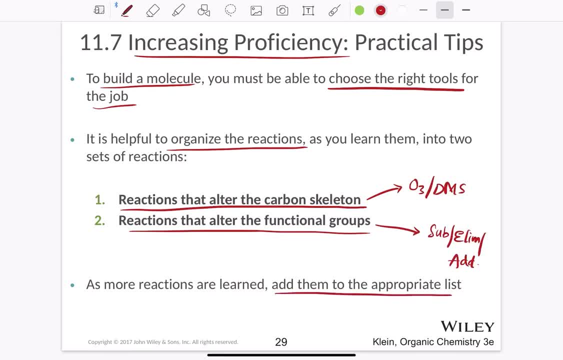 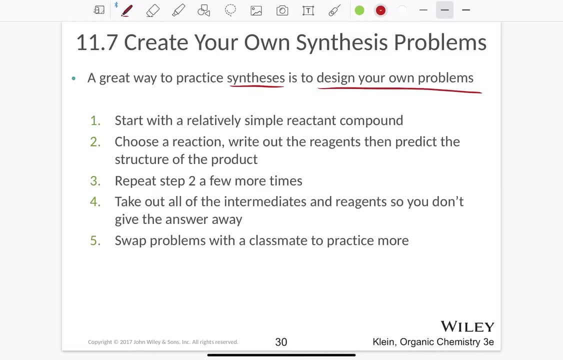 So as you learn more and more reactions, we can add them to the appropriate list. So a great way to practice synthesis is to design your own problem. So first process of designing your own synthesis problem: Start with a relatively simple reactant compound. 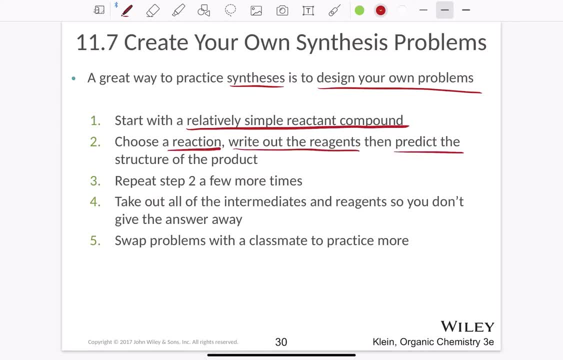 Next, choose a reaction, write out the reagents, then predict the structure of the product And repeat the step a few more times. Take out all the intermediates and reagents so you don't need to give the answer again And swap the problems with a classmate to practice more and more again.